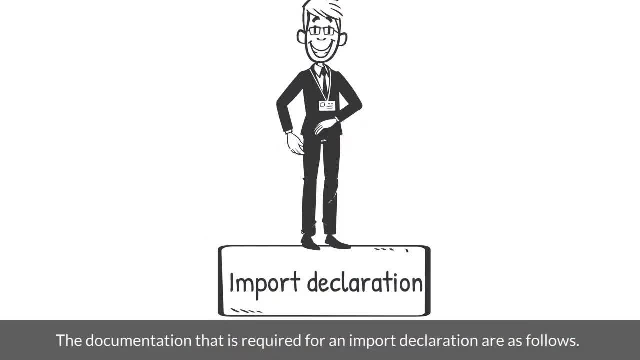 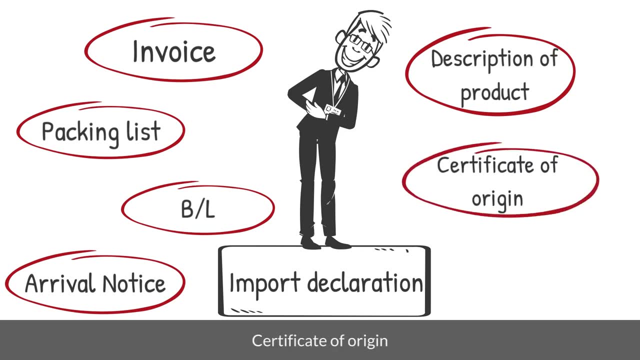 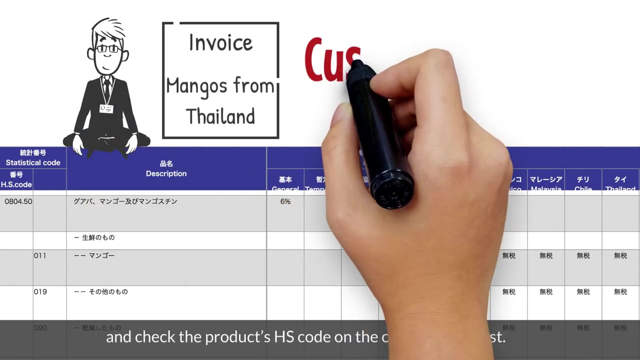 documentation that is required for an import declaration are as follows: invoice packing list- BL arrival notice. description of product certificate of origin, legal permit, if required to import cargo. you need to prepare documentation and send it to a customs specialist. a customs specialist will take a look at the invoice and check the products. HS code on the customs tariff. 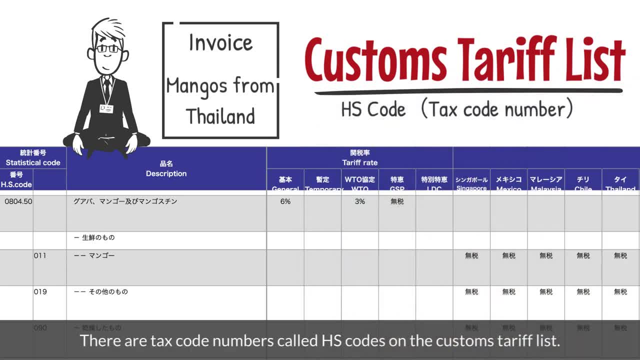 list. there are tax code numbers, called HS codes, on the customs tariff list. nine digits code are allocated for all products. using the list and decide the HS code, then you will check the tax rate. also, EPA is confirmed on the list. for example, when we are importing mangoes to Japan from Thailand, the customs duty is 0% by using EPA. the 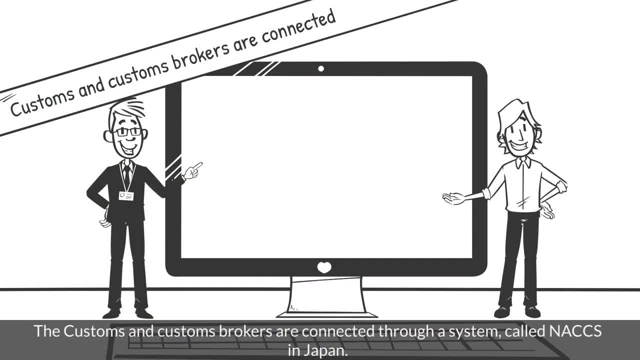 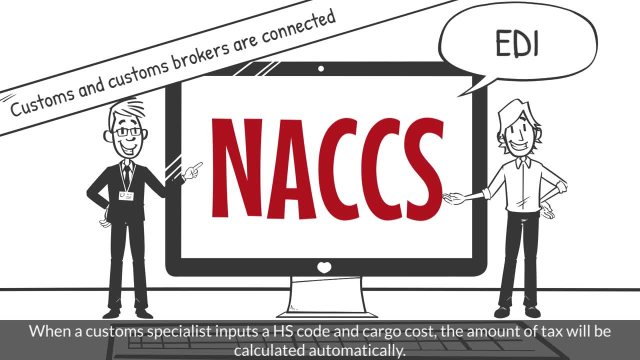 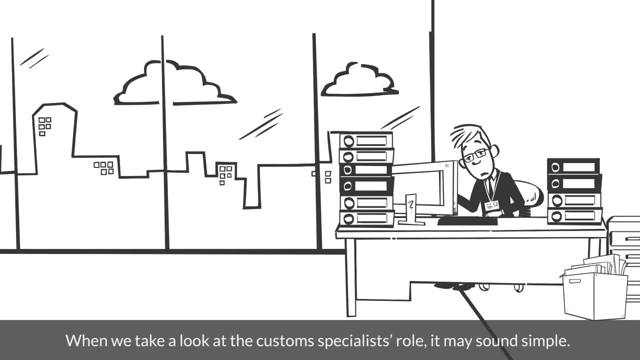 customs and customs brokers are connected through a system called max. in Japan, in Thailand and other countries they called EDI. when a customs specialist and puts a HS code and cargo cost, the amount of tax will be calculated automatically. when we take a look at the customs specialists role, it 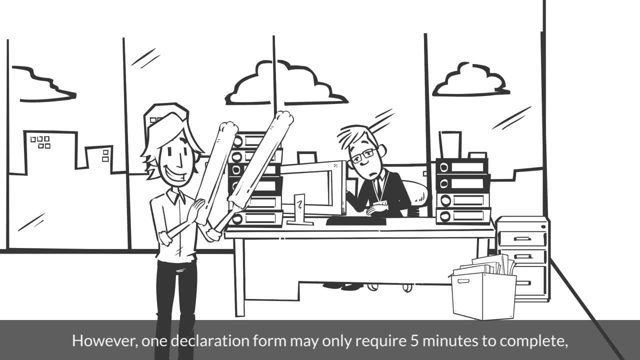 may sound simple. however, one decoration form may only remain in place until the tax is paid, and the tax will be calculated automatically. when we take a look at the customs specialists role, it may sound simple. however, one decoration form may only require five minutes to complete. on the other hand, it may take more than one. 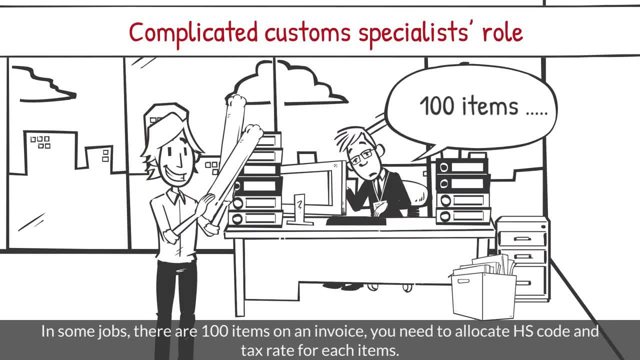 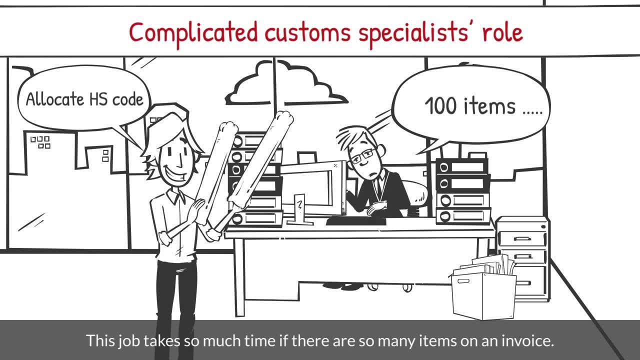 whole day to complete. in some jobs there are 100 items on an invoice. you need to allocate HS code and tax rate for each items. this job takes so much time if there are so many items on an invoice. some items are able to allocate HS code easily, but some items are not so simple to 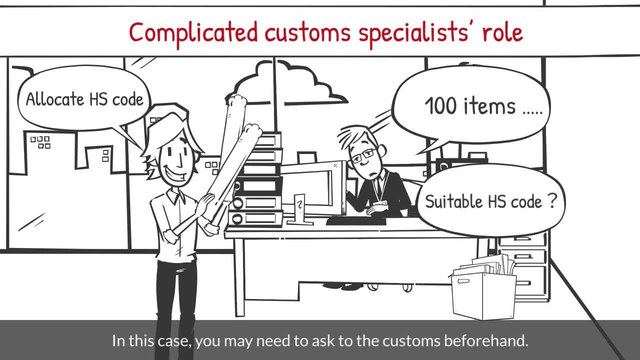 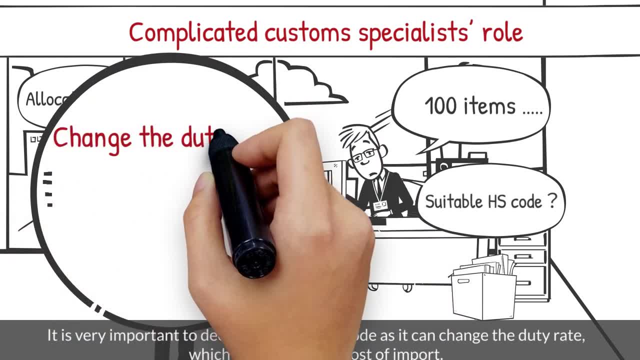 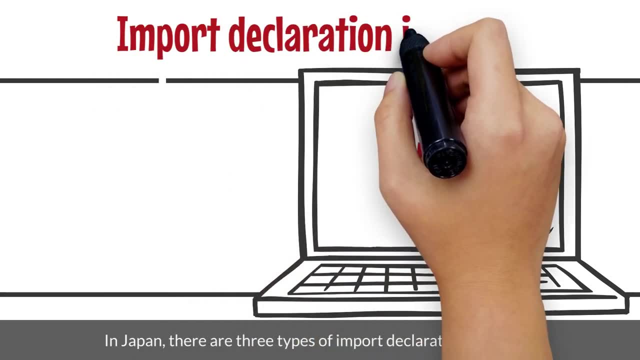 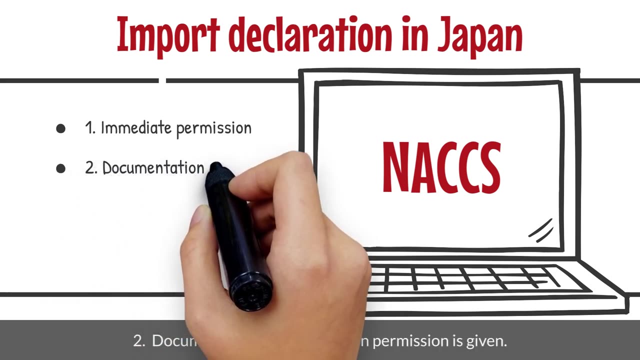 allocate suitable HS code. in this case, you may need to ask to the customs before hand. it is very important to decide a suitable HS code, as it can change the duty rate which may impact the cost of import in Japan. there are three types of import declaration patterns. one: immediate permission is given to documentation. 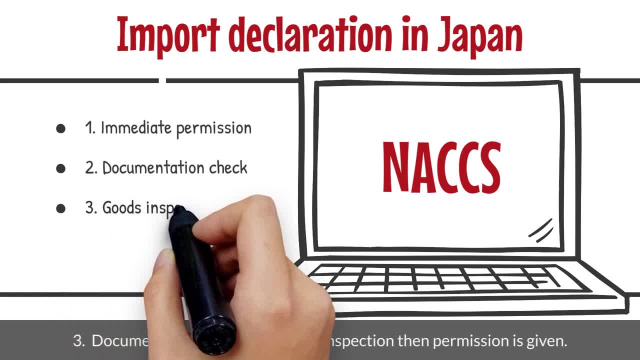 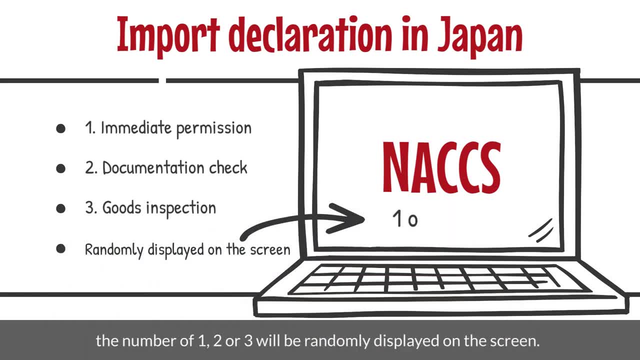 check and then permission is given- three: documentation check and goods inspection. then permission is given once the send button is pressed on, max the number of one, two or three will be randomly displayed on the screen. if one is displayed, the permission is immediate. if two or three is displayed, you need to.